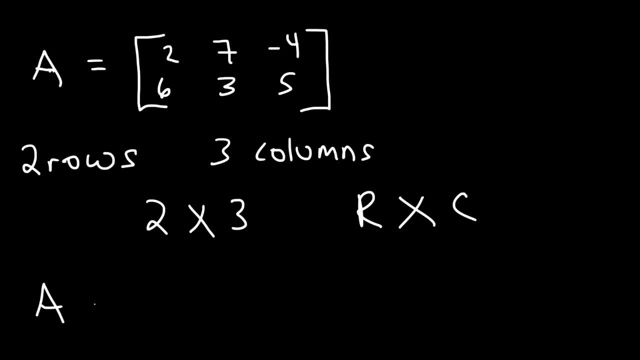 For example, what is element? 2, 3. Or sometimes it can be written as just element A23. So this is in matrix A and the first letter represents the row. The second letter is the column. So this is the first row, this is the second row. This is the first column, second column, third column. So this element, number 5, is in the second row. So this is the first column, second column, third column. So this element, number 5, is in the second row third column. So element A23 has a value of 5. 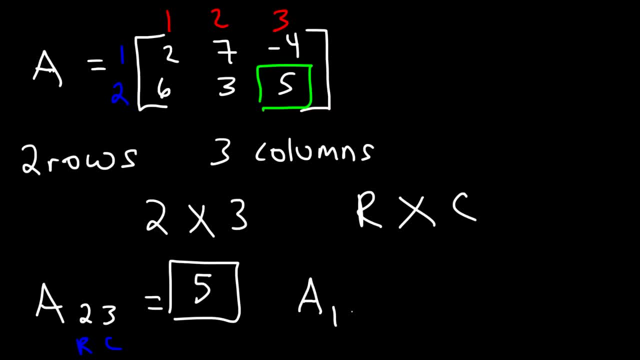 Now here's another one for you. What's element A12 and also element A21? Go ahead and identify the value of these elements. So element A12, that's in the first row, second column. So that has a value of 7. Element A21 is in the second row. So element A21 is in the second row, first column, and so that has a value of 6. Let's consider another matrix. So let's say if we 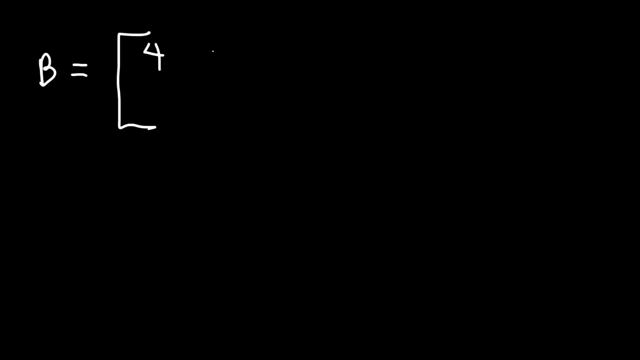 have matrix B, and it has the numbers 4, 3, 7, negative 2, 5, 6, negative 4, 9, negative 3, 8, 1, and negative 7. What is the order of the matrix? So let's start with the rows. 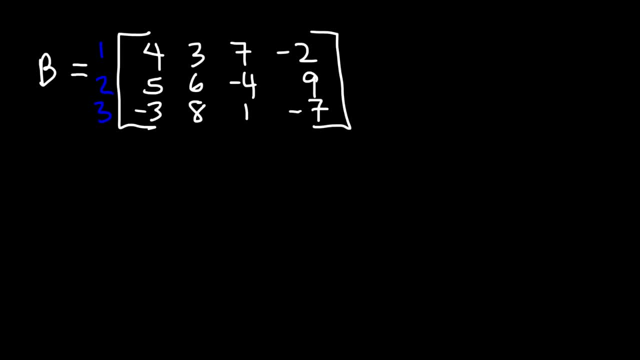 This is row 1, row 2, row 3, and then the columns. Column 1, 2, 3, 4. So the order of matrix B, it's a 3 by 4 matrix. It has 3 rows and 4 columns. 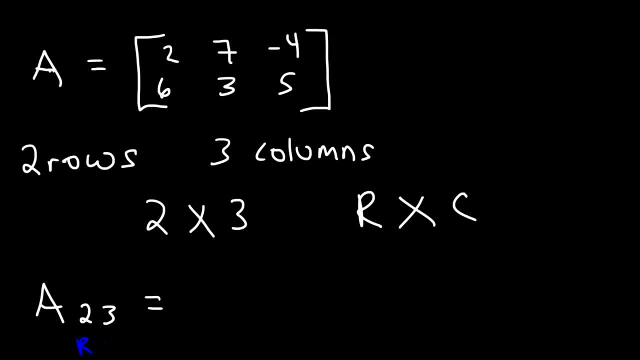 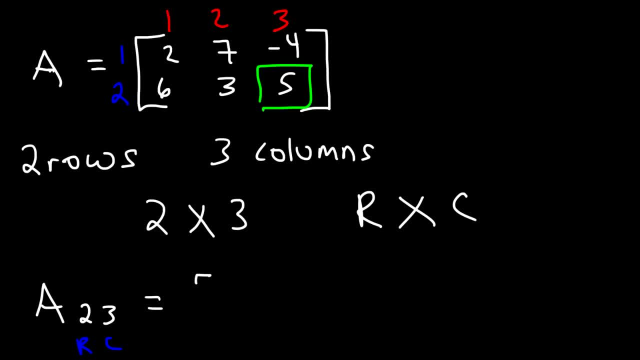 row, third column. So element A23 has a value of 5.. Now here's another one for you. What's element A12 and also element A21? Go ahead and identify the value of these elements. So element A12,, that's in the first row, second column, So that has a value of 7.. Element A21 is in the second. 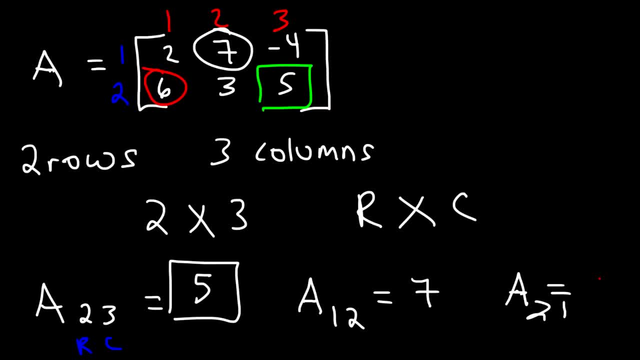 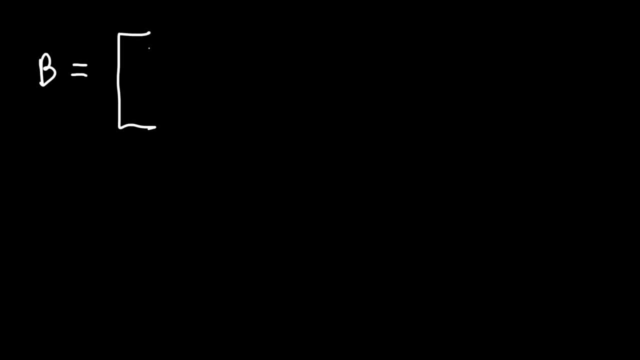 row, first column, And so that has a value of 6.. Let's consider another matrix. So let's say, if we have matrix B and it has the numbers 4, 3, 7, negative 2, 5, 6, negative 4, 9, negative 3,, 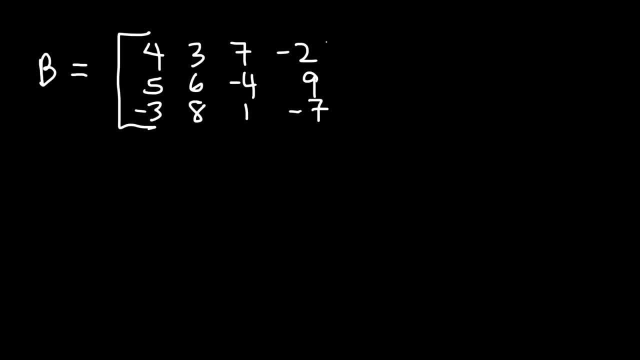 8,, 1, and negative 7.. What is the order of the matrix? So let's start with the row. This is row 1,, row 2, row 3.. And then the columns Column 1,, 2,, 3,, 4.. So the order of 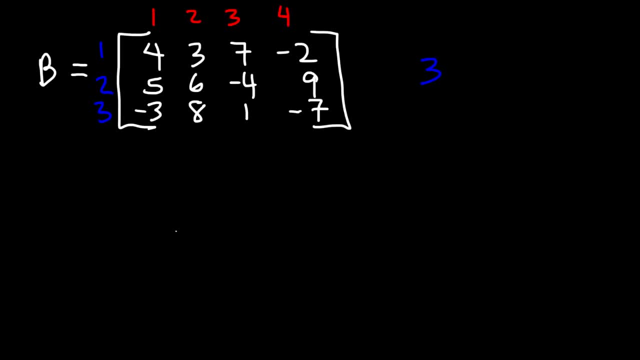 matrix B. it's a 3 by 4 matrix. It has 3 rows and 4 columns. Now identify element B11.. B12,, B13,, B14, and B34.. Go ahead and identify these four elements. So this one is in the first. 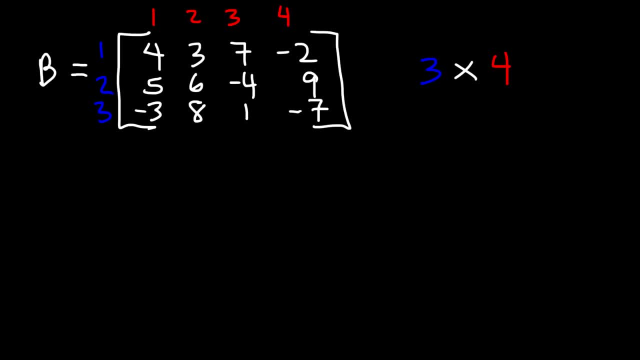 Now identify elements B11, B23, B14, and B34. Go ahead and identify these four elements. So this one is in the first row, first column, so that has a value of 4 element b23 that is in the second row third column so that has a value of negative 4 and then element b14 is in the first row fourth column so that's equal to negative 2 and element b34 is in the third row fourth column so it has a value of negative 7 so you need to be 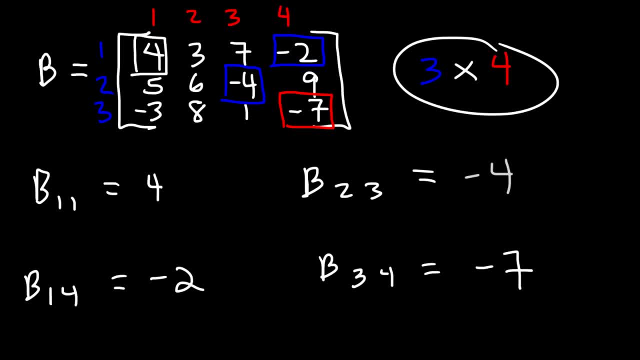 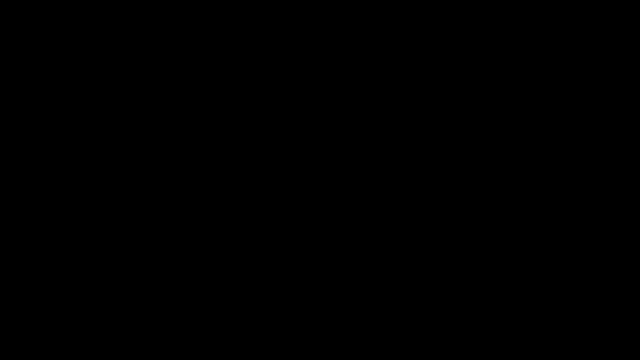 able to determine the order of the matrix and the value of every or any element in the matrix so what I'm going to do at this point is i'm going to give you a list of matrices and I want you to identify the order of each matrix so let's say if we have matrix C and it has a number 3 negative 5 to negative 1 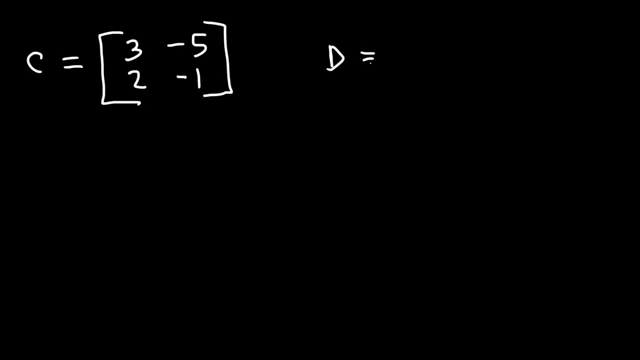 And then we have matrix D, which contains the elements 4, 5, negative 2, 7, 3, and negative 6. 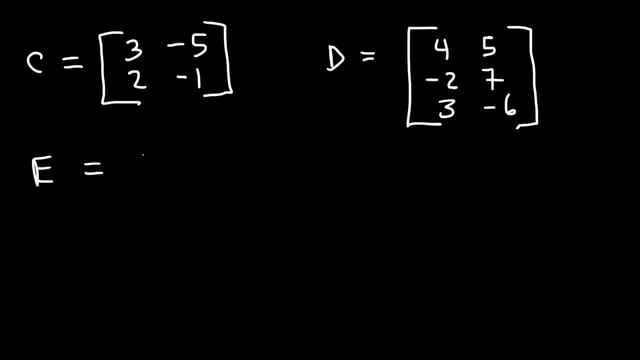 And then we have matrix E, which contains one number, which is 8. And then we have matrix F, which contains 7, 4, negative 5, and 11. 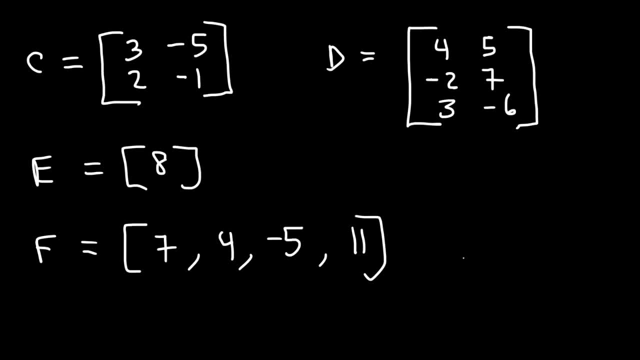 And let's say matrix G has the numbers 3, 1, 7, 2, 6, negative 4, 9, 0, 3. 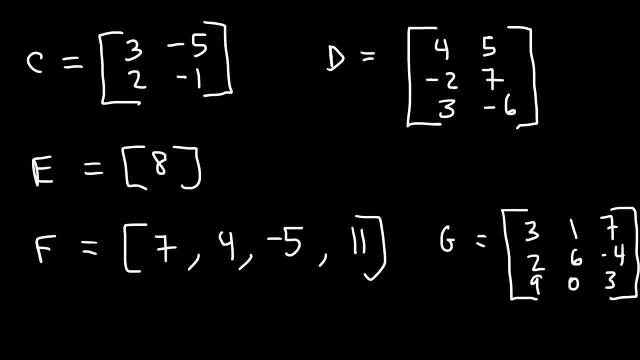 So identify... Identify the order of each matrix. Go ahead and try that. Let me just give you one more. 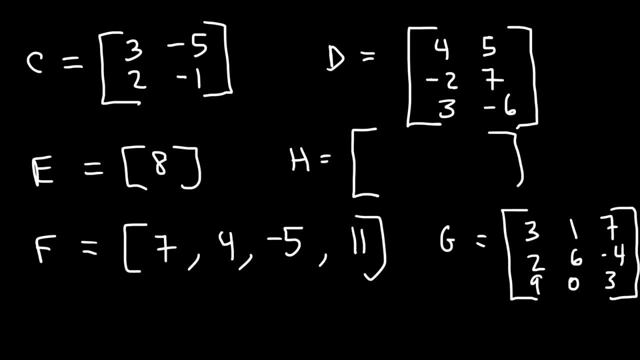 Matrix H, which is going to be 2, 1, 7, negative 3, 6, negative 2, 5, and 4. 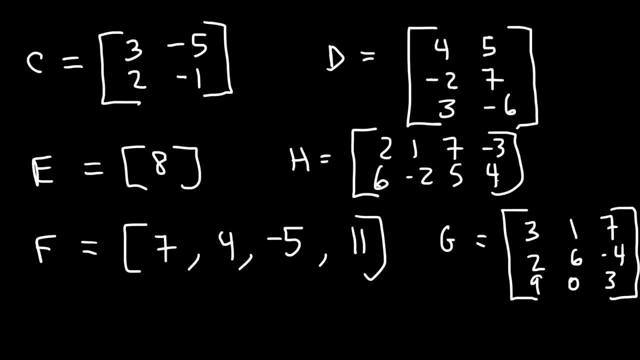 And also determine which of these matrices represents a square matrix. 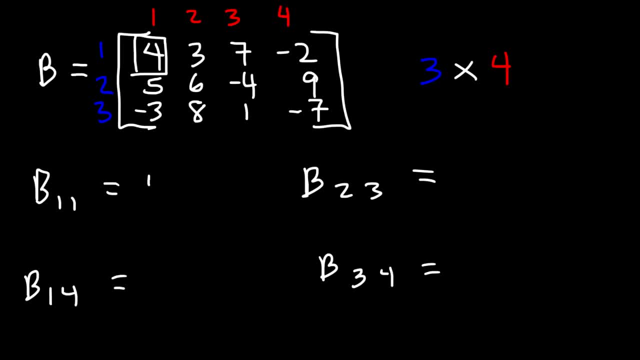 row, first column, So that has a value of 4.. Element B23, that is in the second row, third column, So that has a value of negative 4.. And then element B14 is in the first row, fourth column. 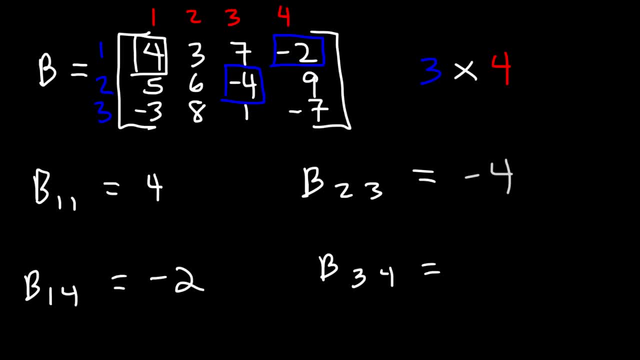 So that's equal to negative 2. And element B34 is in the third row, fourth column, So it has a value of negative 7. So you need to be able to determine the order of the matrix and the value of every or any element in the matrix. 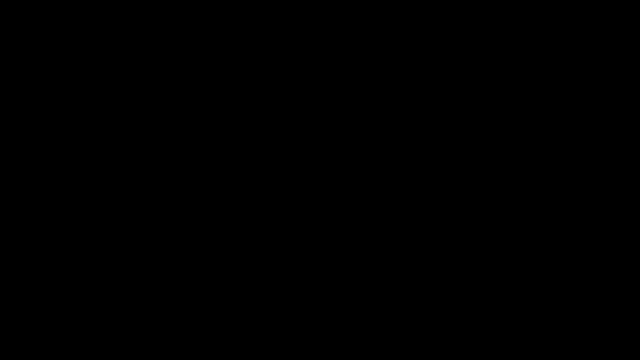 So what I'm going to do at this point is I'm going to give you a list of matrices And I want you to identify the order of each matrix. So let's say, if we have matrix C and it has the numbers 3, negative 5, 2, negative, 1.. And then we have matrix D, which contains the elements. 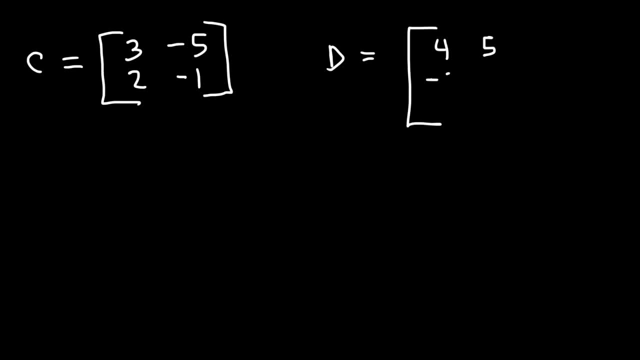 4,, 5, negative 2,, 7,, 3, and negative 6.. And then we have matrix E, which contains one number, which is 8.. Matrix F is going to have 7,, 4, negative 5, and 11.. 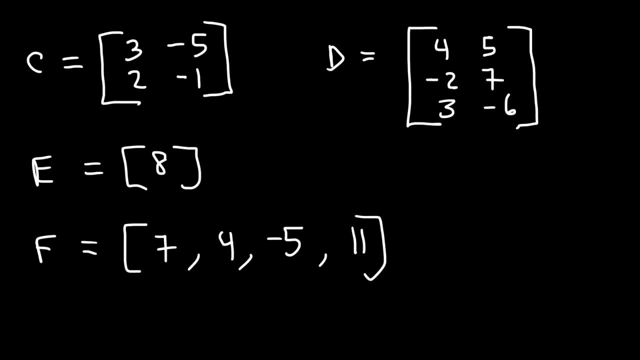 And let's say matrix G has the numbers 3,, 1,, 7,, 2,, 6, negative 5.. And let's say matrix F has a number 4,, 5,, 1,, 6, negative 5.. And then let's say matrix S has the numbers 3,, 1,, 7,, 2,, 6,, negative 5.. And then let's say matrix C has the elements 2, 6, negative 5,, 2, 6, and negative 6.. 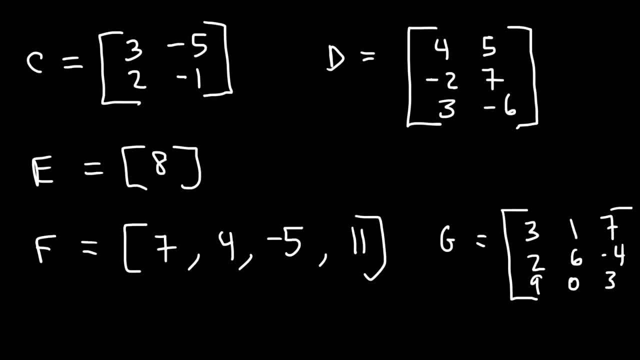 four, nine zero three. so identify the order of each matrix. go ahead and try that. let me just give you one more, matrix H, which is going to be two, one, seven negative three, six negative two, five and four, and also determine which of these matrices represents a square matrix. so let's start with matrix C. it 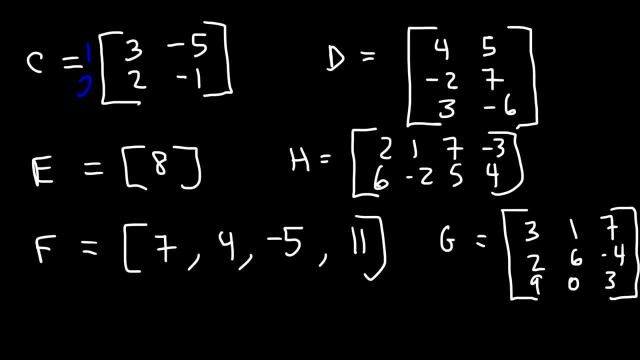 So let's start with matrix C. It's a square matrix. It's a square matrix. It has two rows, and it has two columns. 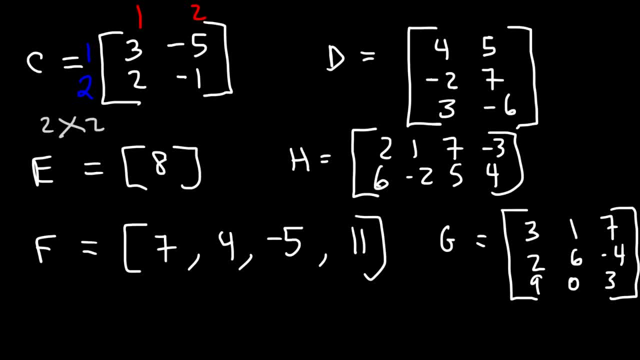 So therefore, it's a 2 by 2 matrix. Now, this is a square matrix because the number of rows and columns are the same. In a square, all sides are the same. 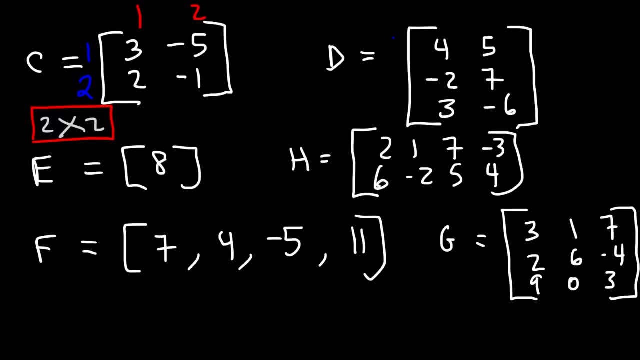 Now, for matrix D, we have three rows and two columns. So this is going to be considered a 3 by 2. 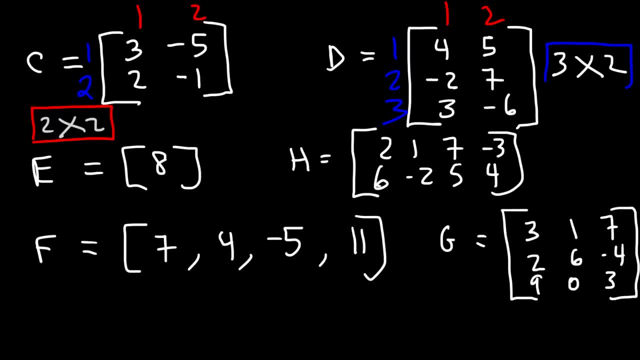 So the order of the matrix is always going to be the number of rows times the number of columns. Now, for matrix E, it has one row and one column. 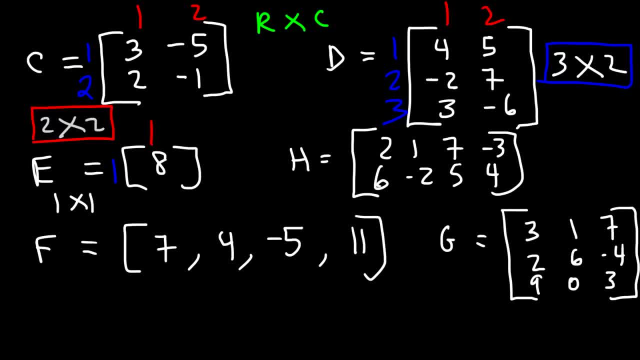 So because it only has one number, it's a 1 by 1 matrix. 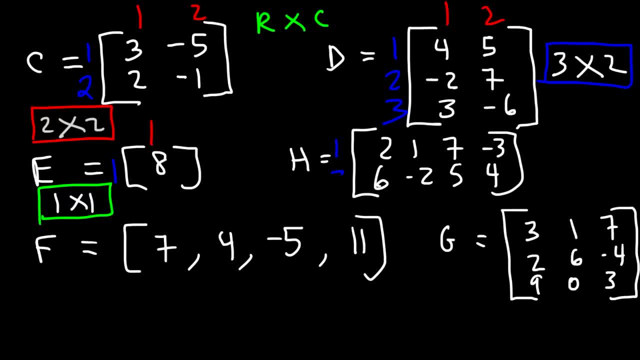 Now, for H, there are two rows and there's three columns. So the order of the matrix is always going to be the number of rows times the number of columns. So this is a 2 by 4 matrix. 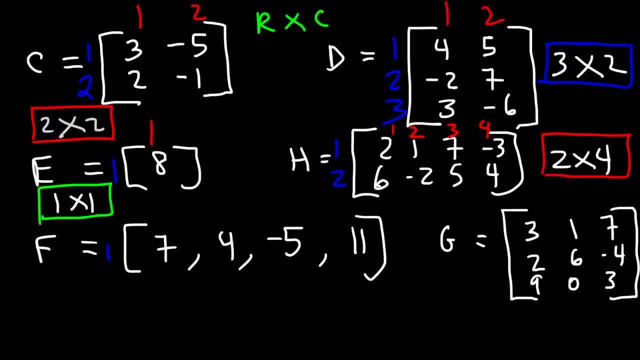 And then for F, we have one row and there's four columns. So that's a 1 by 4 matrix. And finally, the last one, G. That's another square matrix. 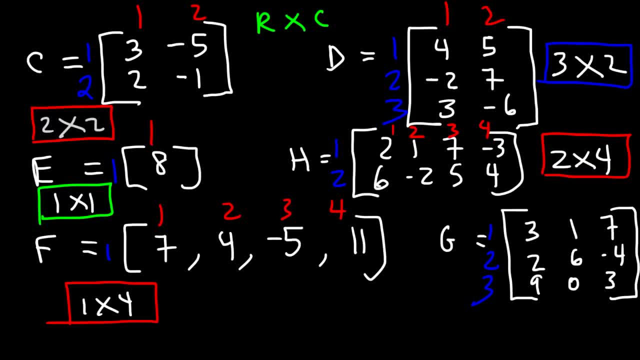 As we can see, there's three rows and it has three columns. So that's a 3 by 3 matrix. 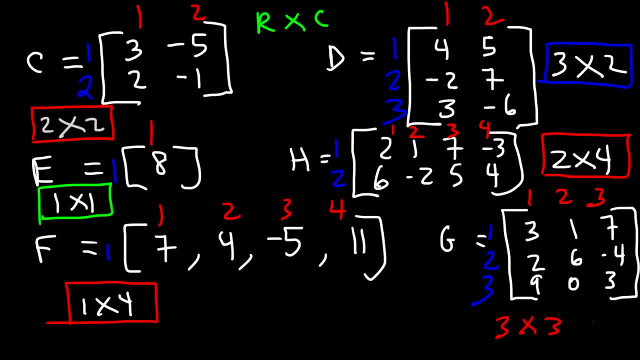 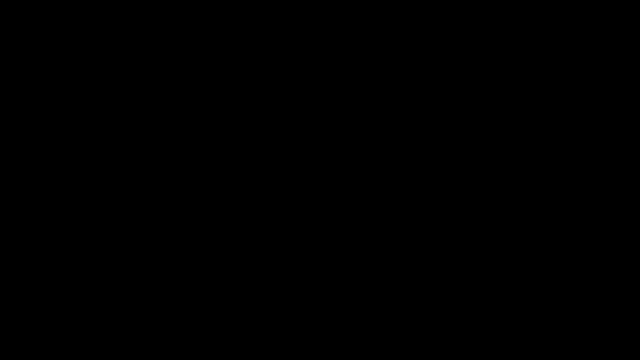 So now you know how to determine the order of the matrix and you also know how to identify the elements within a matrix. 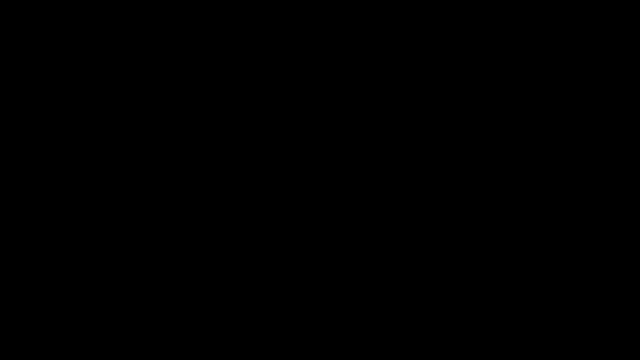 Now let's focus on adding matrices. So let's say if we have matrix A, and it has the numbers 2, 3, 5, negative 4, and we have 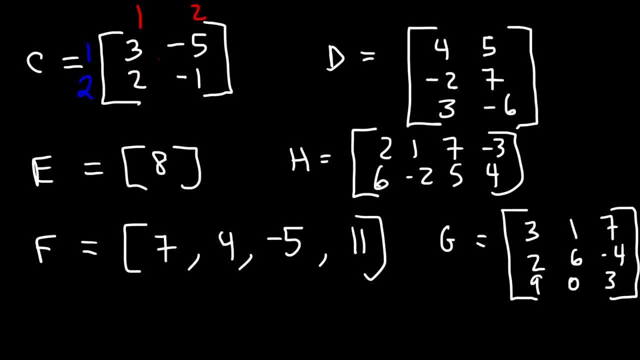 has two rows and it has two columns, so therefore it's a 2 by 2 matrix. now, this is a square matrix because the number of rows and columns are the same and the square- all sides are the same. now for matrix D, we have three rows and two columns, so this is going to be considered a 3x2 matrix. so 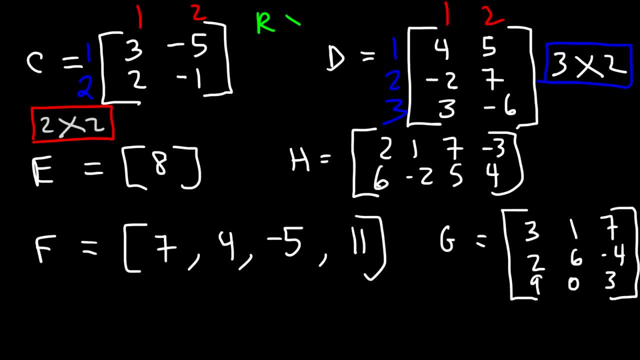 the order of the matrix is always going to be the number of rows times the number of columns. now for matrix E. it has one row and one column, so because it only has one number, it's a one-by-one matrix. now for H, there are two rows and there's four columns, so this is a 2x4 matrix, and 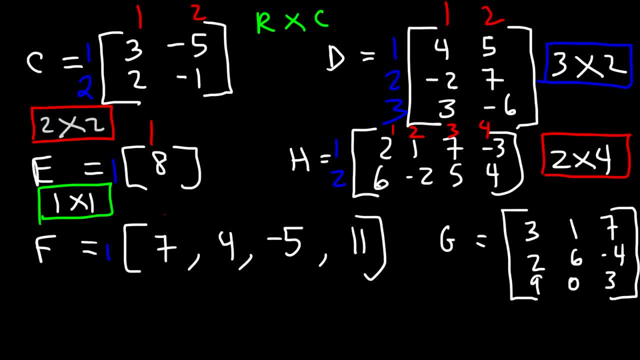 then for F, we have one row and there's four columns, so that's a 1x4 matrix. and finally the last one, G, that's another square matrix. as we can see, there's three rows and it has three columns, so that's a 3x3 matrix. so now you know how. 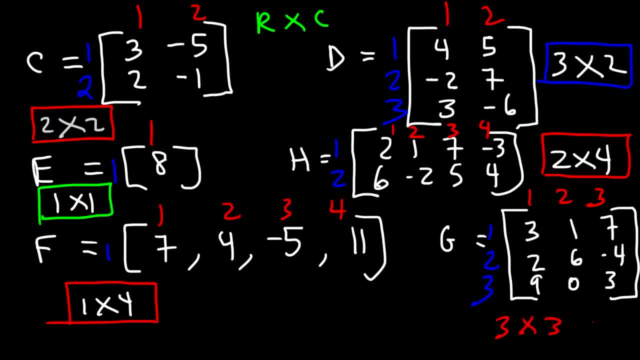 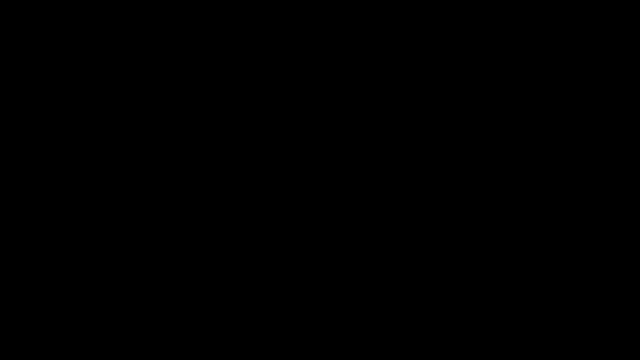 to determine the order of the matrix and you also know how to identify the elements within a matrix. now let's focus on adding matrices. so let's say, if we have matrix A and it has the numbers 2, 3, 5, negative 4, and we have matrix B and 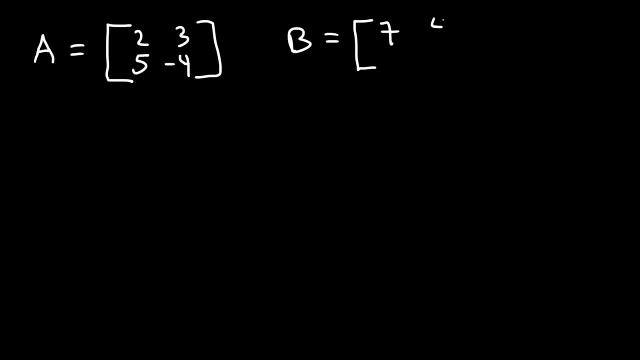 which is 7, 4 negative, 3 and 5. what is the sum of matrix A and B? so for add in those two matrices, all we need to do is add the corresponding elements and, by the way, if you have a 2x2 matrix, you can only add it to another 2x2 matrix. 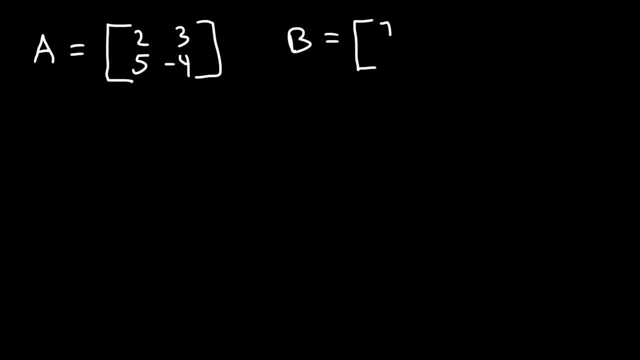 matrix B, which is 7, 4, negative 3, and 4. So let's say we have matrix A, and it has the numbers 2, 3, 5, negative 4, and we have matrix B, which is 7, 4, negative 3, and 4. So now let's do matrix A. 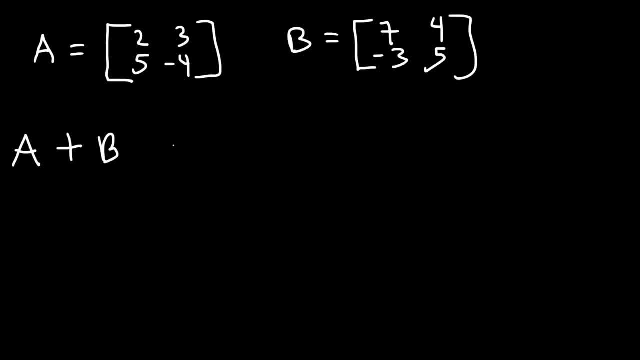 What is the sum of matrix A and B? So if we're adding those two matrices, all we need to do is add the corresponding elements. And by the way, if you have a 2 by 2 matrix, you can only add it to another 2 by 2 matrix. The number of rows and columns must be the same when adding matrices. So the first element, the one in the first row, first column, we need to add it with element B11 in the first row and the first column, they have to match. So this is going to be 2 plus 7, and then we need to add these two. So in the first row, second column, it's going to be 3 plus 4, and then we're going to add those two numbers. 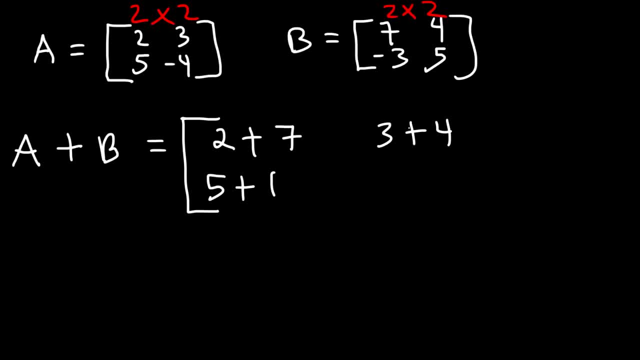 So that's going to be 5 plus negative 3, and these two numbers, which are in the second row, second column, the result will remain in that position, second row, second column. 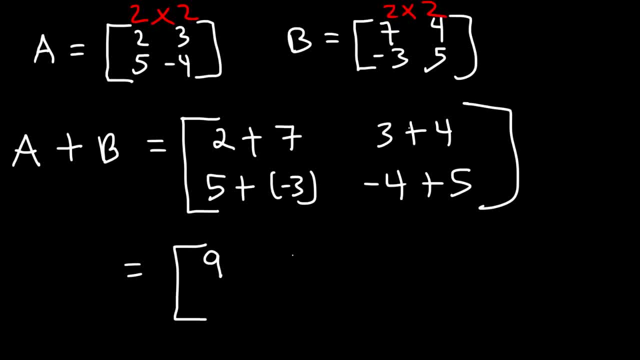 Now 2 plus 7 is 9, 3 plus 4 is 7, 5 plus negative 3 is 2, negative 4 plus 5 is 1. So this is the sum of matrix A and B. 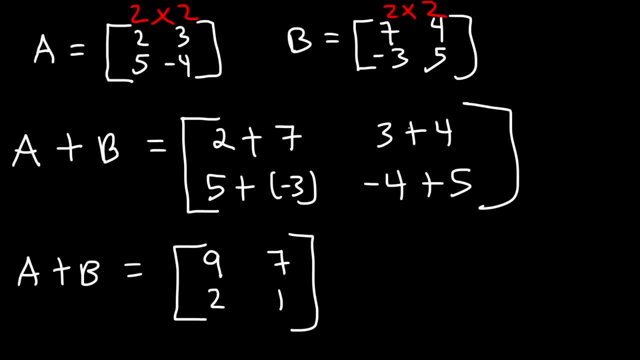 And that's a simple way to add two matrices together. It's not very complicated. 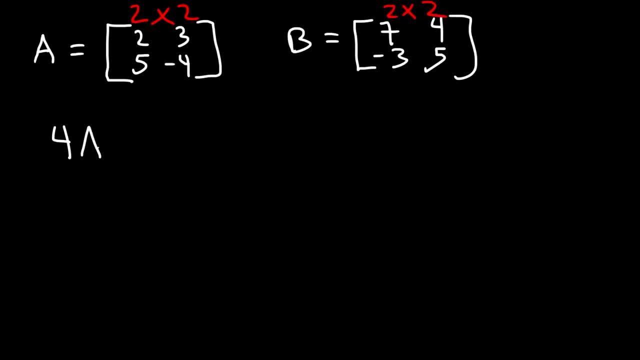 Now let's say if you want to multiply matrix A by 4, what will you get? 4 times A, all you need to do is multiply every element by 4. So it's going to be 4 times 2, 4 times 3, 4 times 5, and 4 times 7. 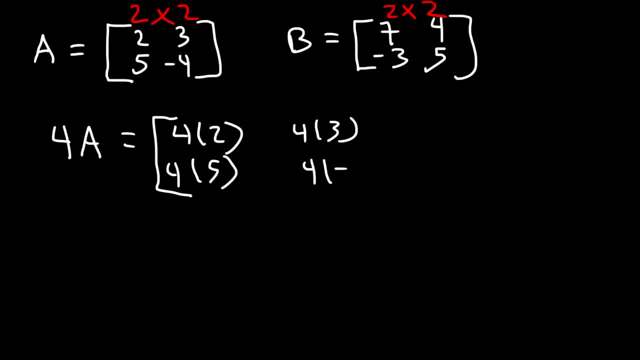 So that's going to be 4 times 2, 4 times 3, 4 times 5, and 4 times 7. So that's going to be 4 times 2, 4 times 3, 4 times 7. So that's going to be 4 times negative 4. So then 4A is going to equal 8, 12, 20, and negative 16. 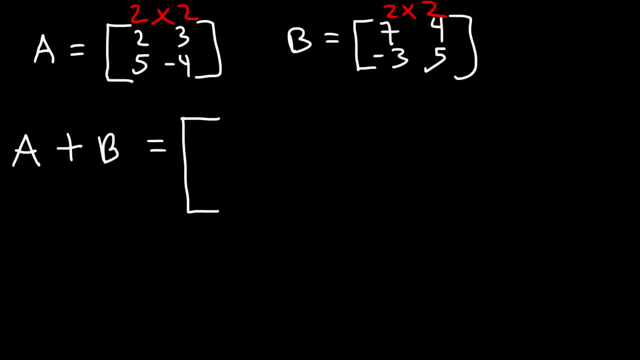 the number of rows and columns must be the same when adding matrices or subtracting matrices as well. so the first element, the one in the first row, first column, we need to add it with element B 1: 1 in the first row, in the first column. they have to. 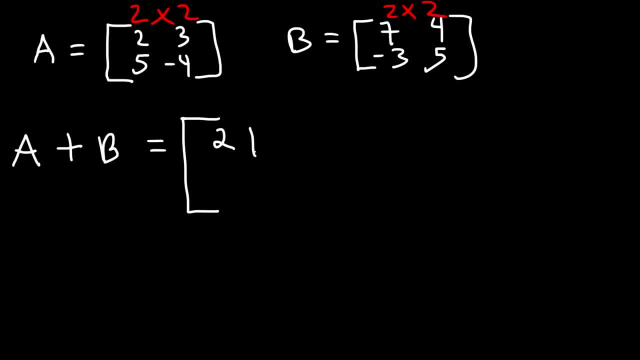 match. so this is going to be 2 plus 7 and then we need to add these two. so in the first row, second column, is going to be 3 plus 4 and then we're going to add those two numbers, so that's going to be 5 plus negative 3, and these two numbers, which are 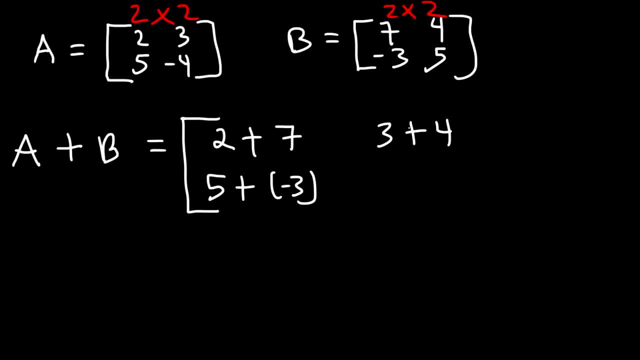 in the second row, second column. the result will remain in that position. second row, second column. now: 2 plus 7 is 9. 3 plus 4 is 7. 5 plus negative: 3 is 2. negative 4 plus 5 is 1. 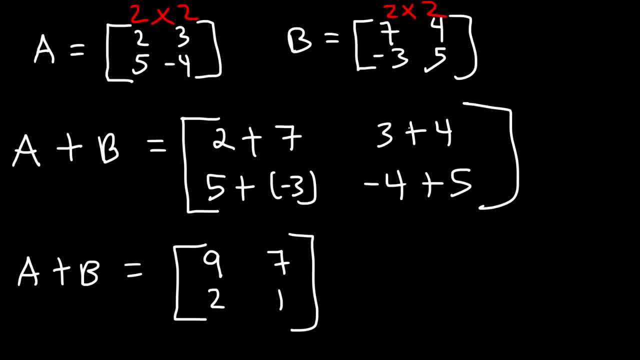 matrix A and B, And that's a simple way to add two matrices together. It's not very complicated. Now let's say: if you want to multiply matrix A by 4, what will you get? 4 times A? all you need to do is multiply every element by 4.. So it's. 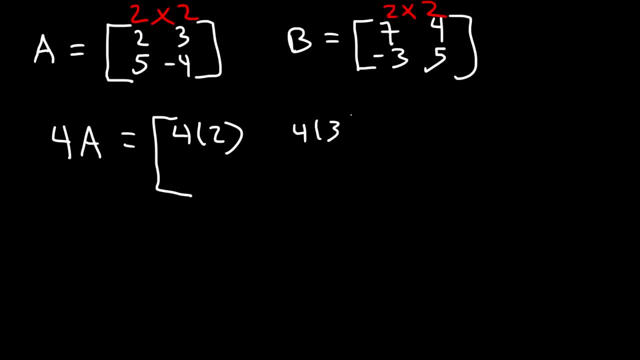 going to be 4 times 2,, 4 times 3,, 4 times 5, and 4 times negative 4.. So then, 4A is going to equal 8,, 12,, 20, and negative 16.. 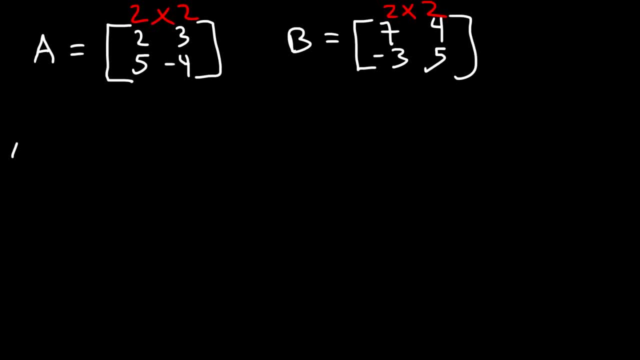 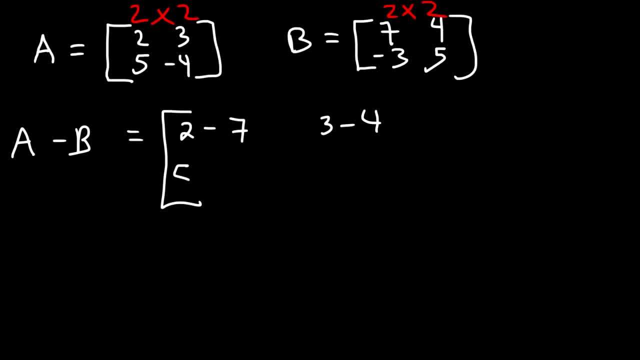 minus 7,, 3 minus 4,, 5 minus negative 3, and then negative 4 minus 5.. So A minus B, that's going to be 2 minus 7,, which is negative 5.. 3 minus 4 is negative 1. 5 minus.